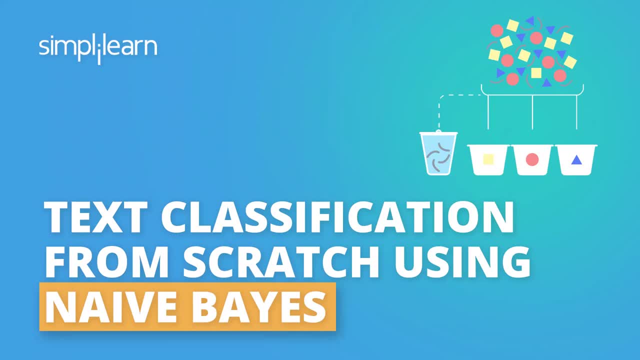 We're going to do the use case text classification Now. I would challenge you to go back and send us a note on the notes below underneath the video and request the data for the shopping cart So you can plug that into Python code and do that on your own time so you can walk through it, since we walked through all the information on it. But we're going to do a Python code doing text classification- Very popular for doing the naive bays. So we're going to use our new tool to perform a text classification of news headlines and 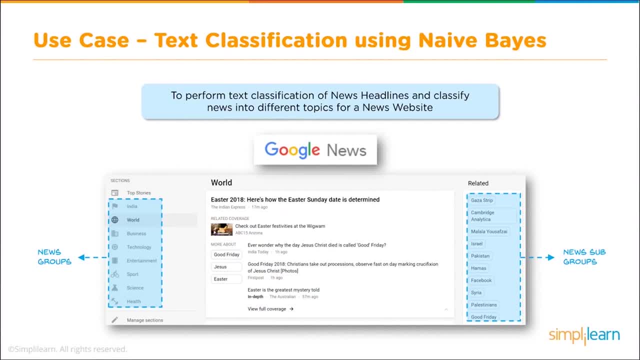 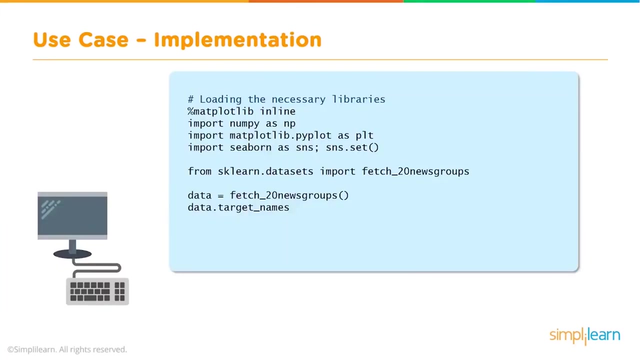 classify news into different topics for a news website. As you can see here we have a nice image of the Google News and then related on the right subgroups. I'm not sure where they actually pulled the actual data we're going to use from. It's one of the standard sets, But certainly this can be used on any of our news headlines and classification. So let's see how it can be done using the naive bays classifier. Now we're at my favorite part. We're actually going to write some Python script, Roll up our sleeves and we're going to start by doing our imports. These are 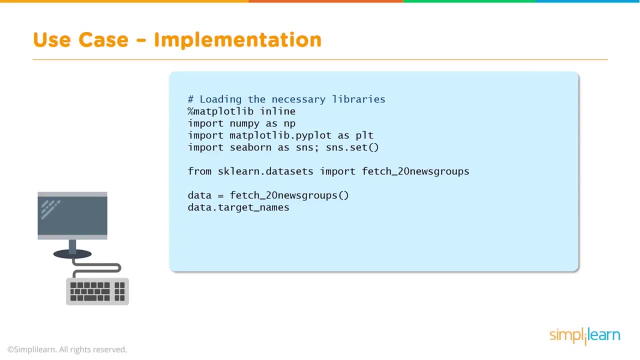 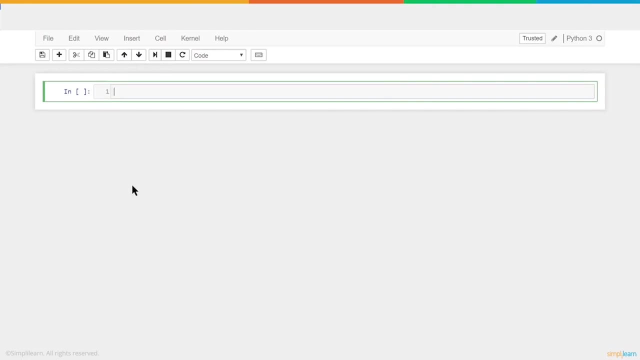 very basic imports, including our news group, And we'll take a quick glance at the target names. Then we're going to go ahead and start training our data set and putting it together. We'll put together a nice graph, because it's always good to have a graph to show what's going on. And once we've trained it and we've shown you a graph of what's going on, then we're going to explore how to use it and see what that looks like. Now I'm going to open up my favorite editor or inline editor for Python. You don't have to use this. You can use whatever your editor that you like, Whatever interface IDE you want This, just 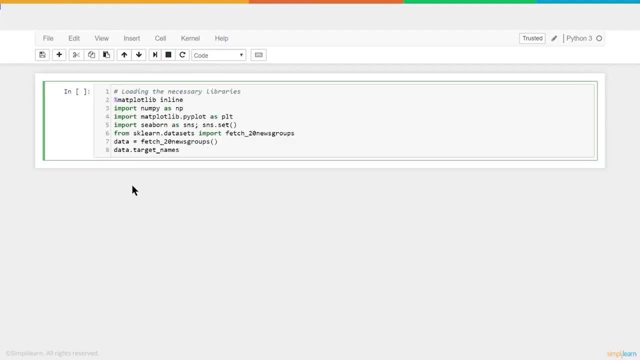 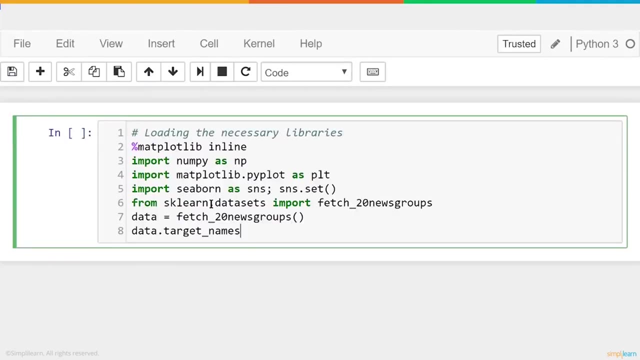 happens to be the Anaconda Jupyter notebook And I'm going to paste that first piece of code in here so we can walk through it. Let's make it a little bigger on the screen so you have a nice view of what's going on. And we're using Python 3. In this case 3.5.. So this would work in any of your 3x. If you have it set up correctly, it should also work in a lot of the 2x. You just have to make sure all of the versions of the modules match your Python version And in here you'll notice the first line is your percentage matplot library inline. Now 3x. 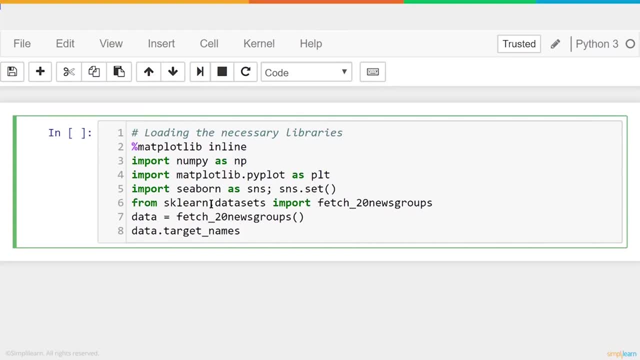 of these lines of code are all about plotting the graph. This one lets the notebook notes- and this is an inline setup- that we want the graphs to show up on this page. Without it, in a notebook like this, which is an explorer interface, it won't show up. Now, a lot of IDEs don't require that. A lot of them- like if I'm working on one of my other setups, it just has a pop up and the graph pops up on there. So you have that setup also. But for this we want the matplot library inline And then we're going to 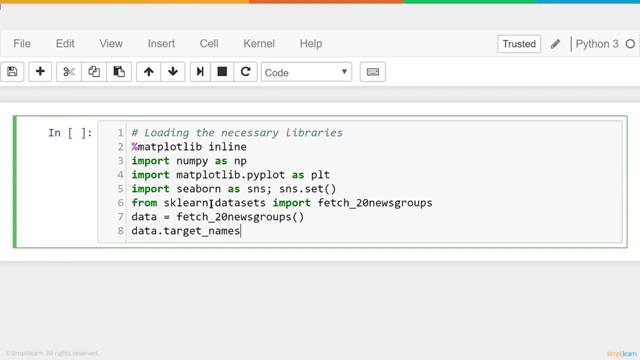 import numpy as np. That's number Python, which has a lot of different formulas in it that we use for both of our sklearn module And we also use it for any of the upper math functions in Python, And it's very common to see that as np, Numpy as np. The next two lines are all about our graphing. Remember I said three of these were about graphing. Well, we need our matplot library, dot pyplot as plt, And you'll see that plt is a very common setup, as is the sns and just like the np. 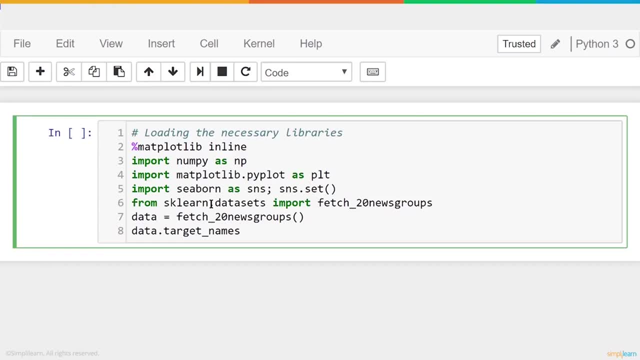 And we're going to import seaborn as sns And we're going to do the snsset. Now, seaborn sits on top of pyplot and it just makes a really nice heatmap. It's really good for heatmaps And if you're not familiar with heatmaps, that just means we give it a color scale. The term comes from the brighter red it is, the hotter. it is in some form of data And you can set it to whatever you want And we'll see that later on. So you'll see that those three lines of code here are just importing the graph function so we can graph it. And as a data scientist, 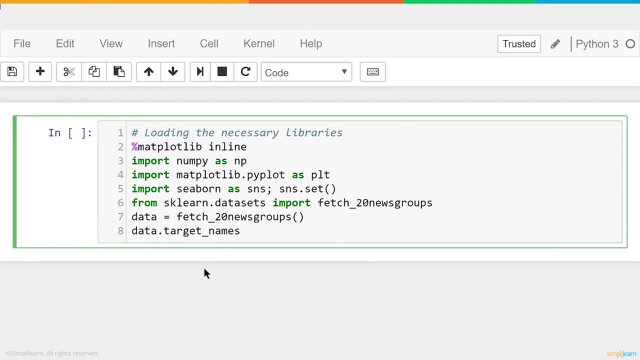 you always want to graph your data and have some kind of visual. It's really hard just to shove numbers in front of people and they look at it and it doesn't mean anything. And then from the sklearndatasets we're going to import the fetch20newsgroups- Very common one for analyzing, tokenizing words and setting them up and exploring how the words work and how do you categorize different things when you're dealing with documents. And then we set our data equal to fetch20newsgroups, So our data variable will have the data in it And we're going to go ahead and just print the target. 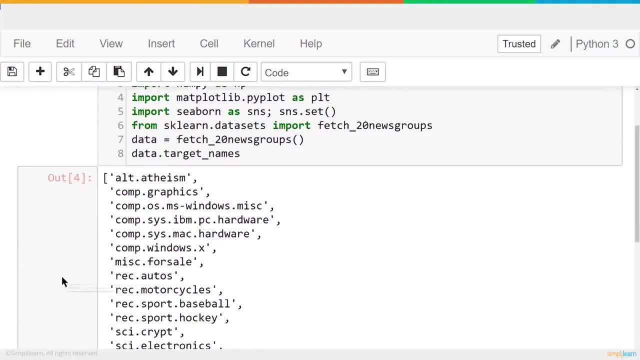 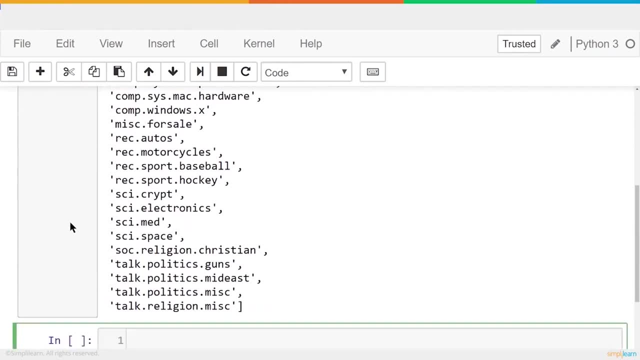 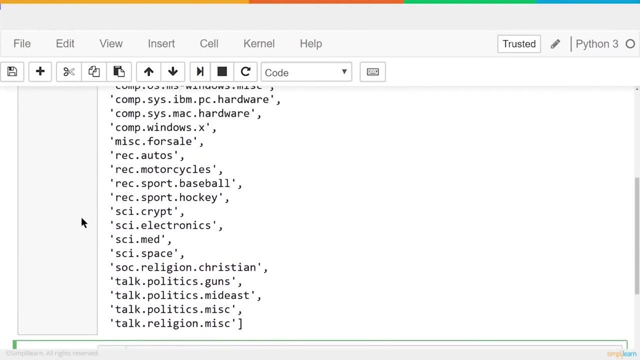 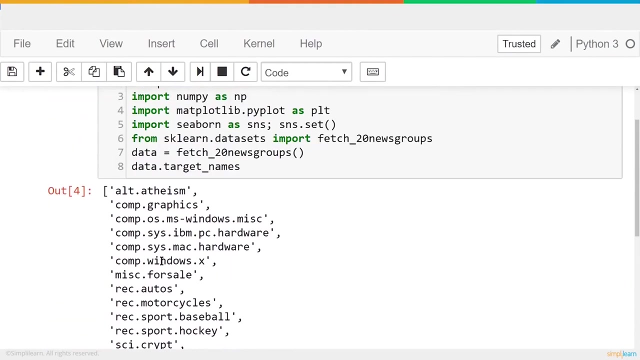 names, Datatargetnames, And let's see what that looks like And you'll see, here we have alt, atheism, comp graphics, comp os, ms windowsmiscellaneous, And it goes all the way down to talkpoliticsmiscellaneous, talkreligionmiscellaneous. These are the categories they've already assigned to this newsgroup And it's called fetch20 because you'll see, there's- I believe there's- 20 different topics in here, or 20 different categories as we scroll down. Now we've gone through the 20 different categories and we're going to go ahead and 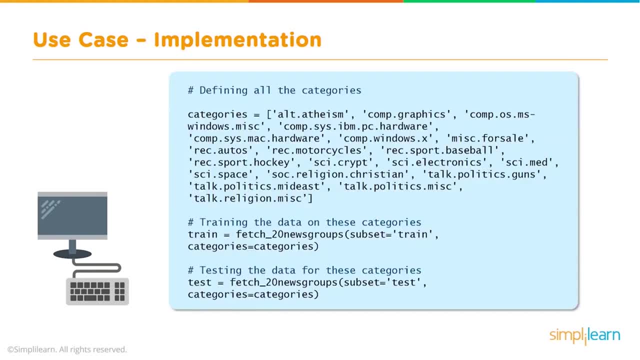 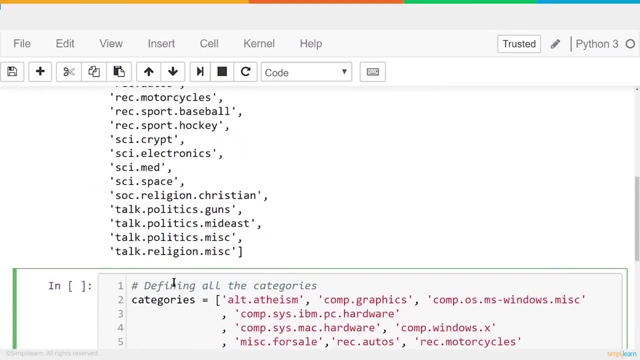 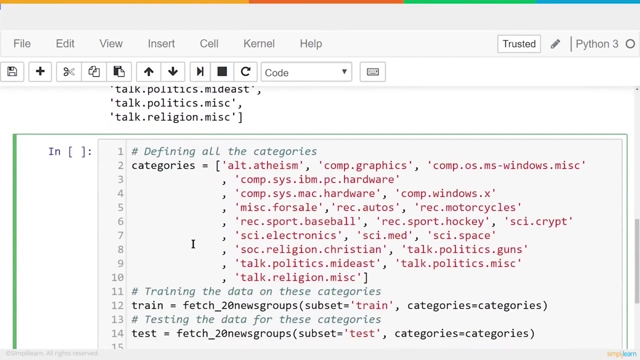 start defining all the categories and set up our data. So we're actually getting here going to go ahead and get the data all set up and take a look at our data And let's move this over to our Jupyter notebook And let's see what this code does. First, we're going to set our categories. Now, if you noticed up here, I could have just as easily set this equal to datatarget underscore names, because it's the same thing. But we want to kind of spell it out for you so you can see the different categories. It kind of makes it more visual so you can see what your data is looking like. 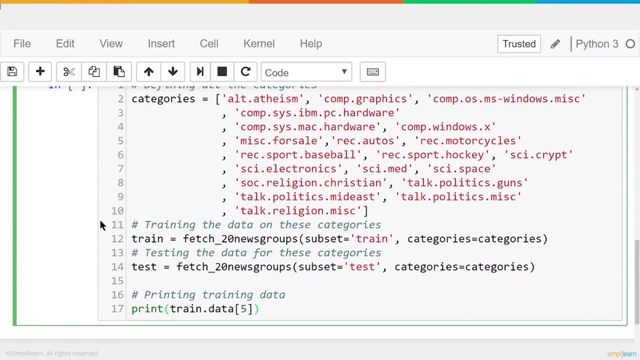 in the background, Once we've created the categories, we're going to open up a train set. So this training set of data is going to go into fetch20 newsgroups and it's a subset in there called train and categories equals categories. So we're pulling out those categories that match And then, if you have a train set, you should also have the testing set. We have test equals fetch20 newsgroups, subset equals test and categories equals categories. Let's go down one size so it all fits on my screen. There we go, And just so we can really see what. 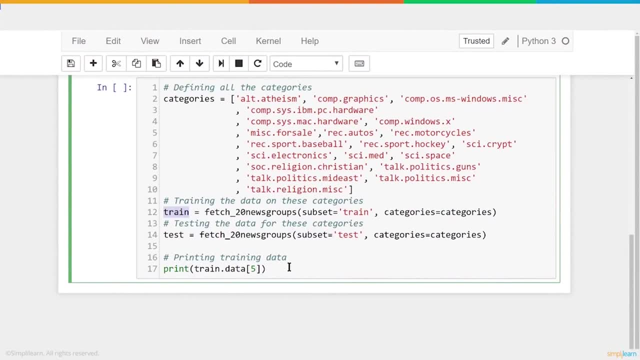 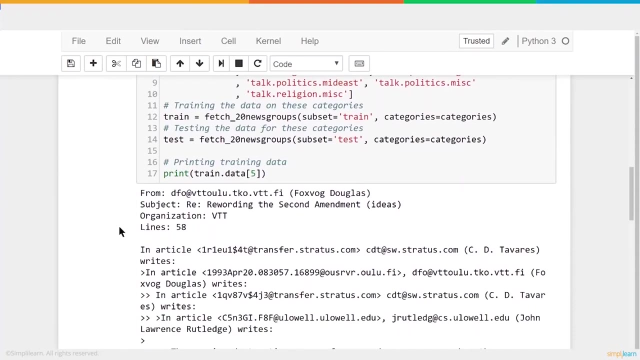 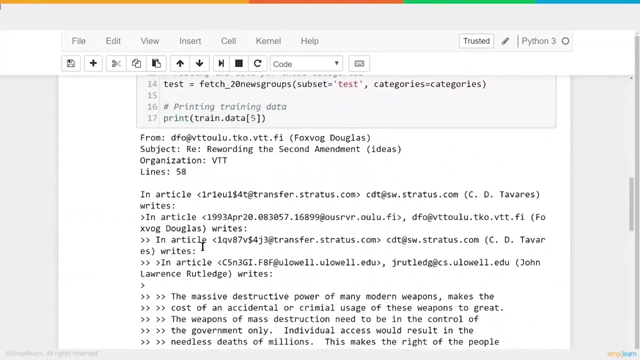 is going on. Let's see what happens when we print out one part of that data. So it creates train and under train it creates train dot data. And we're just going to look at data piece number five And let's go ahead and run that and see what that looks like. And you can see, when I print train dot data number five under train, it prints out one of the articles. This is article number five. You can go through and read it on there And we can also go in here and change this to test, which should look identical, because it's splitting the data. 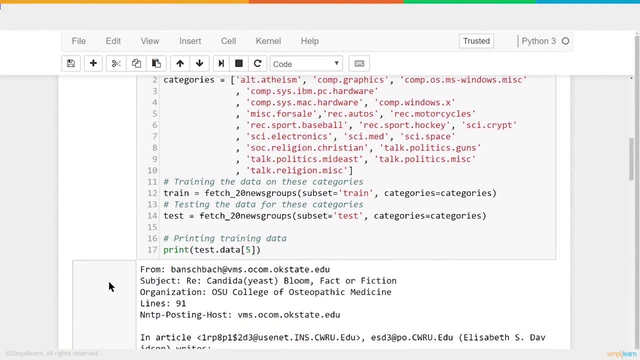 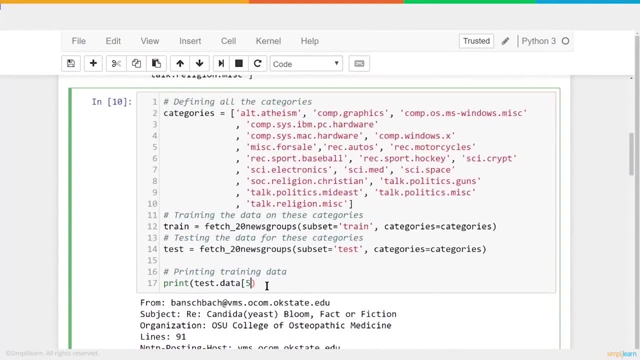 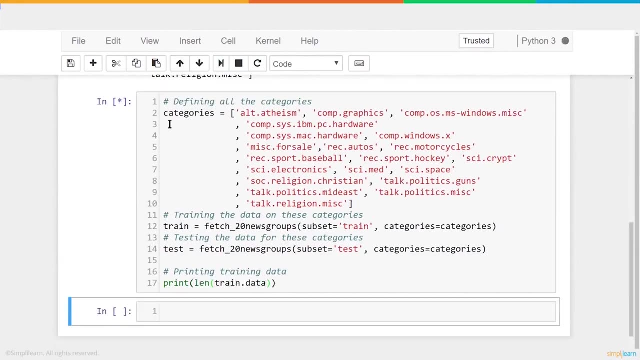 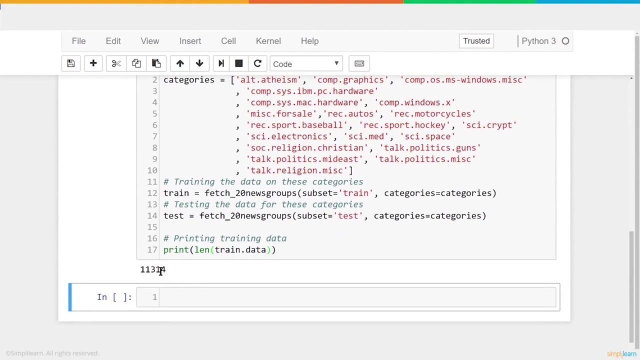 into different groups: Train and test And we'll see. test number five is a different article but it's another article in here And maybe you're curious and you want to see just how many articles are in here. We could do length of train dot data And if we run that you'll see that the training data has 11,314 articles. So we're not going to go through all those articles. That's a lot of articles, But we can look at one of them just so you can see what kind of information is coming up. 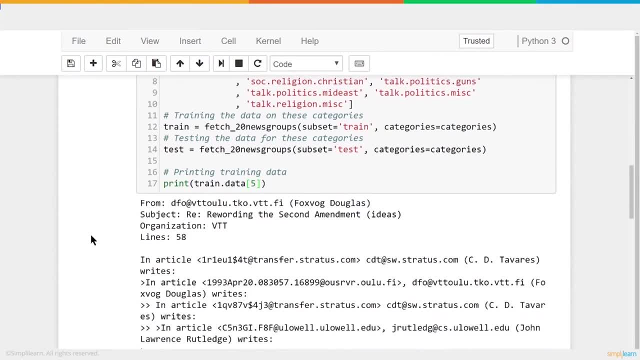 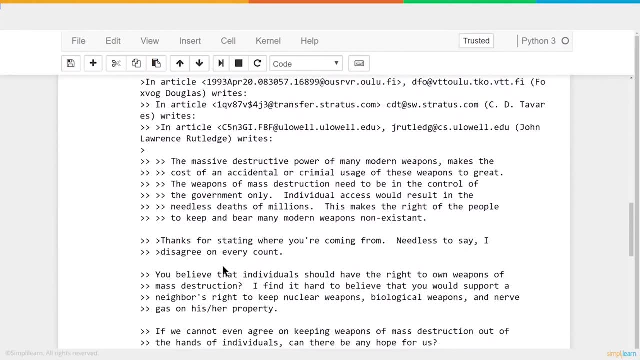 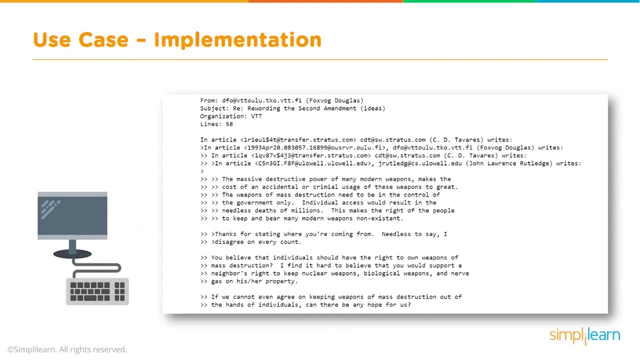 And we'll just look at number five for today. And here we have it, rewording the second amendment, IDs VTT, line 58, lines 58 in article etc. And you can scroll all the way down and see all the different parts to there. Now we've looked at it and that's pretty complicated when you look at one of these articles to try to figure out how do you weight this. If you look down here we have different words and maybe the word from- Well from- is probably in all the articles, so it's not going to have a lot of meaning as far as trying to figure out whether this article fits one of the categories. 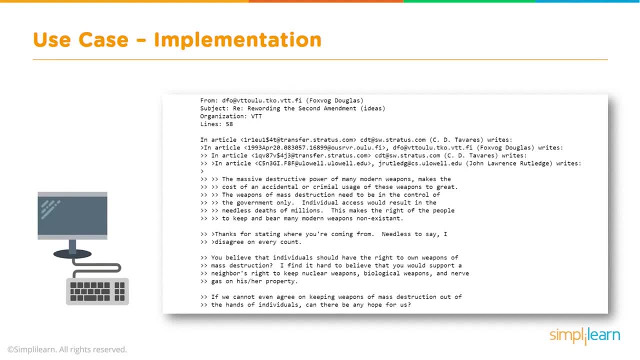 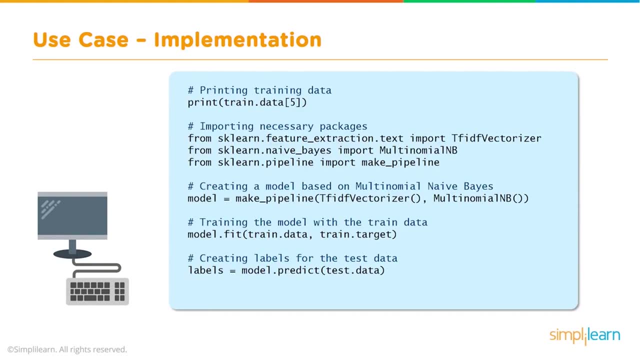 Or not. So trying to figure out which category fits in based on these words is where the challenge comes in. Now that we've viewed our data, we're going to dive in and do the actual predictions. This is the actual naive base, And we're going to throw another model at you or another module at you here in just a second. We can't go into too much detail, But it deals specifically working with words and text and what they call tokenizing those words. So let's take this code and let's skip on over to our Jupiter notebook and walk through it, And here we are. 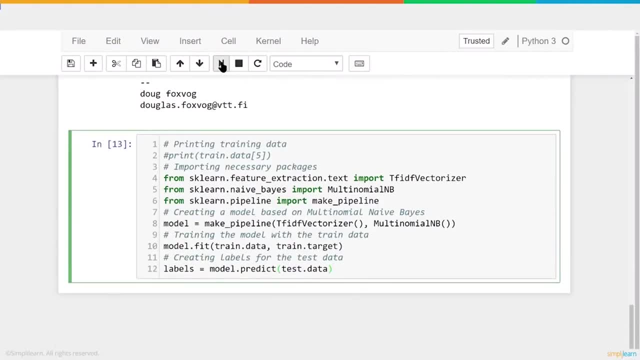 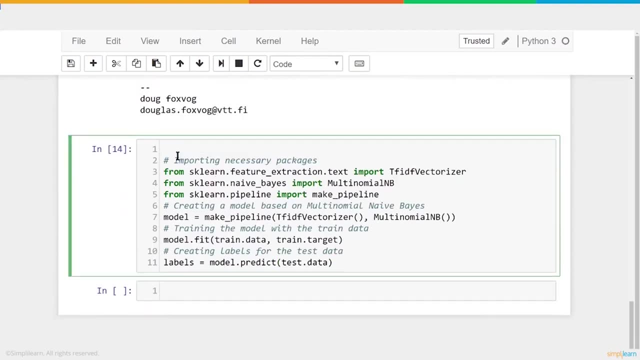 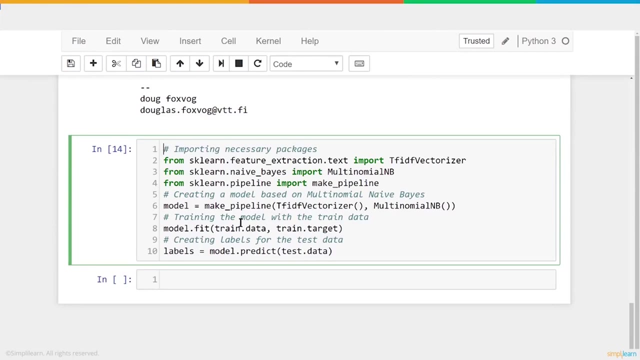 in our Jupiter notebook. Let's paste that in there And I can run this code right off the bat. It's not actually going to display anything yet, But it has a lot going on in here. So the top: we had the print module from the earlier one. I didn't know why that was in there. So we're going to start by importing our necessary packages And from the sklearnfeaturesextractiontxt we're going to import tfidfvectorizer. I told you we're going to throw a module at you. We can't go too much into the math behind this or how it works. You can look it up. 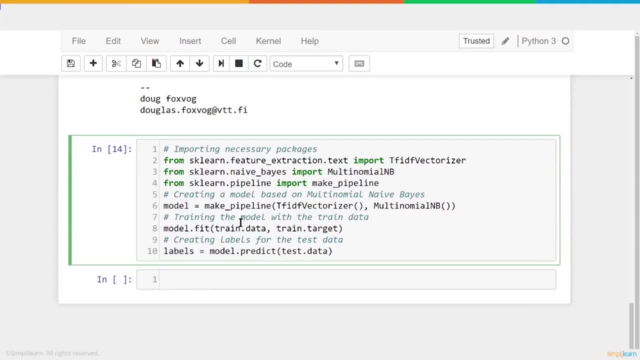 The notation for the math is usually tfidf And that's just a way of weighing the words, And it weighs the words based on how many times they're used in a document, How many times or how many documents they're used in, And it's a well used formula. It's been around for a while. It's a little confusing to put this in here, But let's let it know that it just goes in there and weights the different words in the document for us. That way we don't have to wait, And if you put a weight on it- If you remember I was talking about that up here earlier- If these are 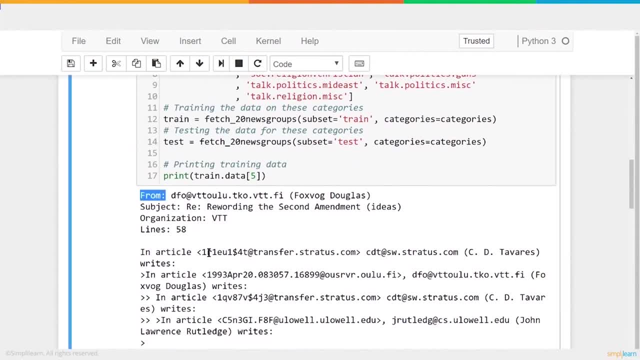 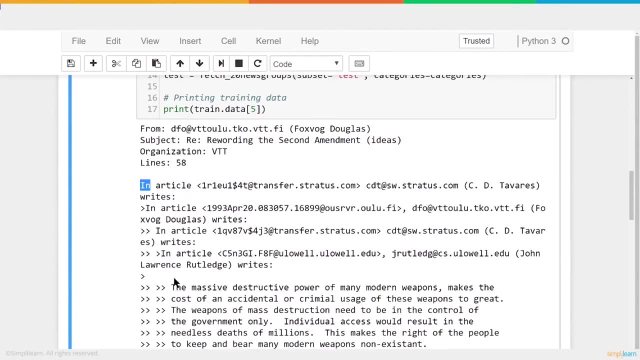 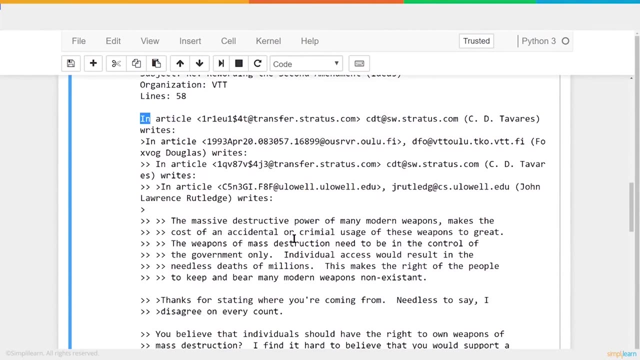 all emails they probably all have the word from in them. From probably has a very low weight. It has very little value in telling you what this document's about. Same with words like in an article, in articles in cost of, on, maybe, cost, might, or where words like criminal weapons, destruction. These might have a heavier weight because they describe a little bit more what the article's doing. Well, how do you figure out all those weights in the different articles? That's what this module does. That's what the tfidfvectorizer is going to do. 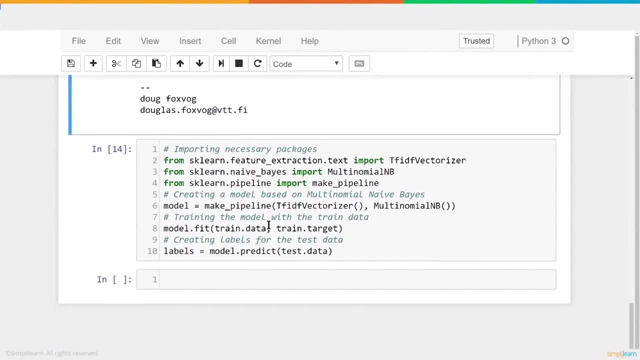 And then we're going to import our sklearnnaivebase And that's our multinomial nb- Multinomial naive base- Pretty easy to understand that Where that comes from. And then finally we have the sklearn pipeline, import make pipeline. Now, the make pipeline is just a cool piece of code Because we're going to take the information we get from the tfidfvectorizer And we're going to pump that into the multinomial nb. So a pipeline is a 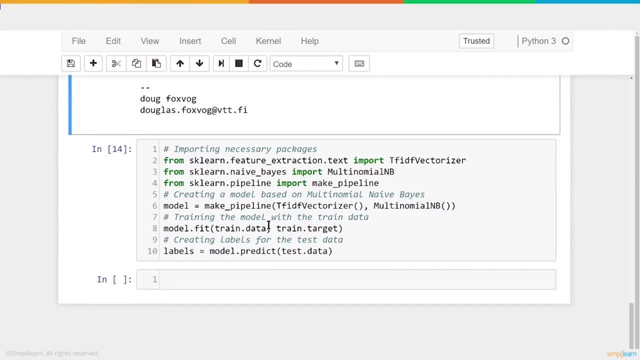 way of organizing how things flow. It's used commonly. You probably already guessed what it is. if you've done any businesses, They talk about the sales pipeline. If you're on a work crew or project manager, You have your pipeline of information that's going through Or your projects and what has to be done in what order. That's all this pipeline is. We're going to take the tfidvectorizer and then we're going to push that into the multinomial nb. Now we've designated that as the variable model. We have our pipeline model. 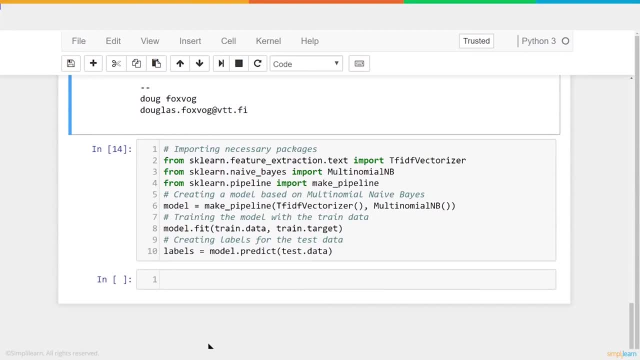 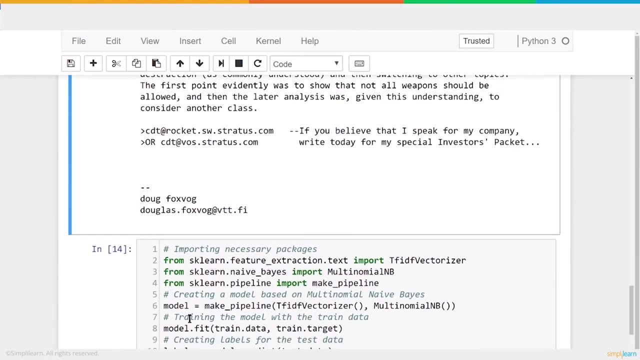 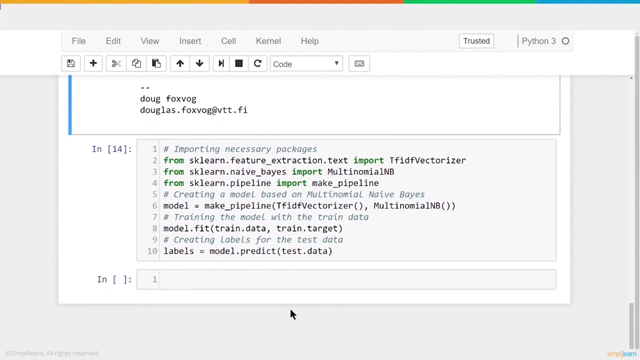 And we're going to take that model And this is just so elegant. This is done in just a couple lines of code- Modelfit- And we're going to fit the data And first the train data And then the train target. Now the train data has the different articles in it- You can see the one we were just looking at And the traintarget is what category they already categorized that particular article as, And what's happening here is the train data is going into the tfidvectorizer. 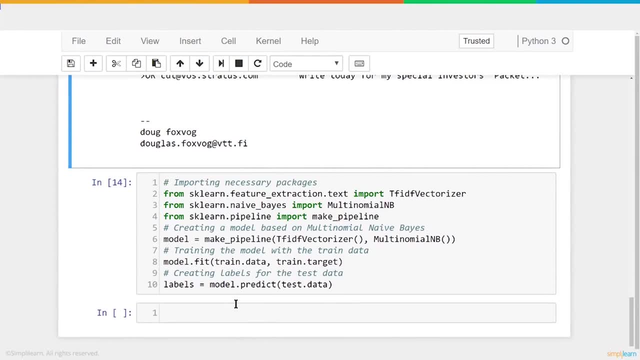 so when you have one of these articles that goes in there, it weights all the words in there. so there's thousands of words with different weights on them. i remember once running a model on this and i literally had 2.4 million tokens go into this. so when you're dealing like large document, 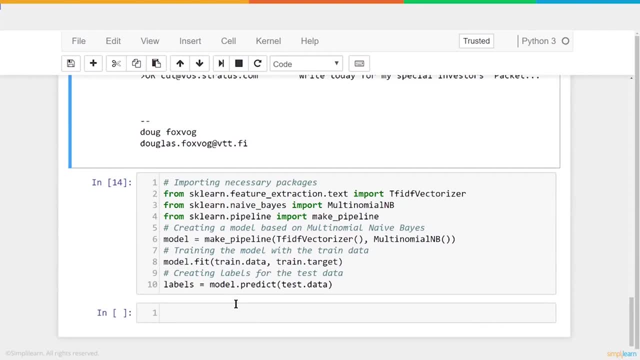 bases, you can have a huge number of different words. it then takes those words, gives them a weight and then, based on that weight, based on the words and the weights, and then puts that into the multinomial nb and once we go into our naive bays we want to put the train target in there. so the 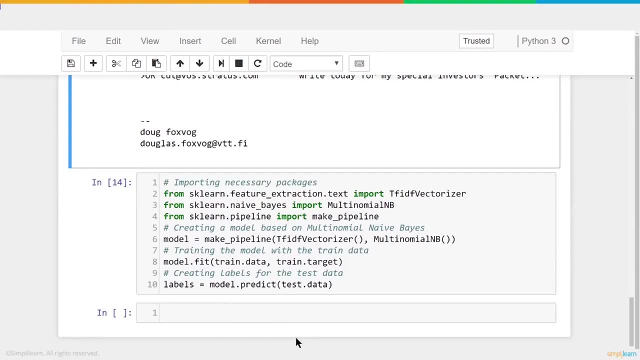 train data that's been mapped to the tfid vectorizer is now going through the multinomial nb. and then we're telling it: well, these are the answers, these are the answers to the different documents. so this document that has all these words, with these different weights from the first part, is going: 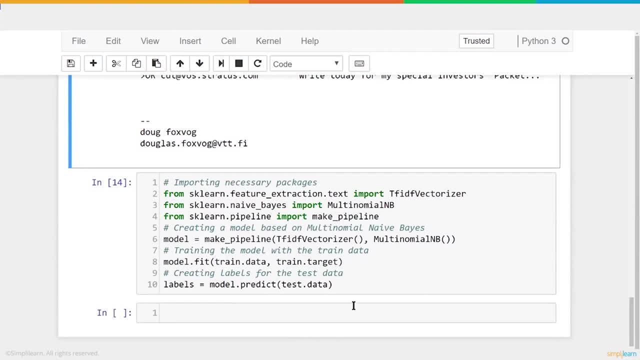 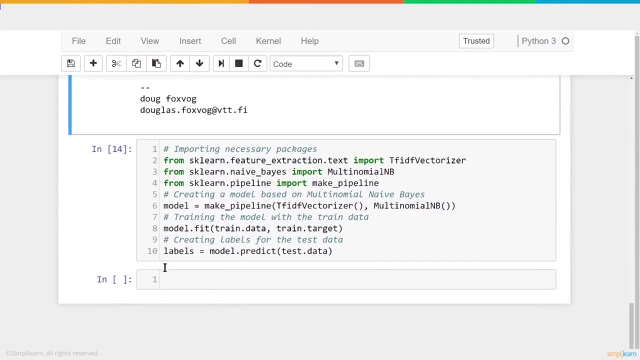 to be, whatever category it comes out of- maybe it's the talk show or the article on religion- miscellaneous. once we fit that model, we can then take labels and we're going to set that equal to model dot predict. most of the sklearn use the term dot predict to let us know that we've now trained. 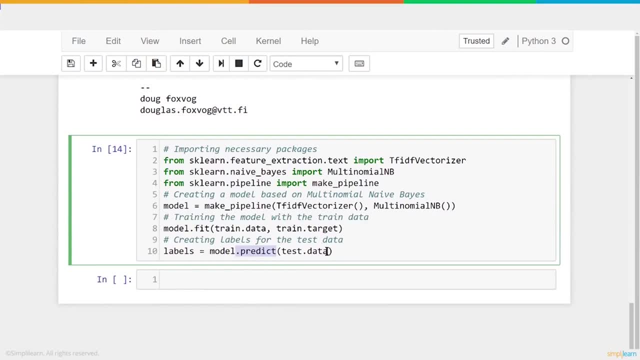 the model, and now we want to get some answers and we're going to put our test data in there, because our test data is the stuff we held off to the side, we didn't train it on there and we don't know what's going to come up out of it, and we just want to find out how good our labels are. 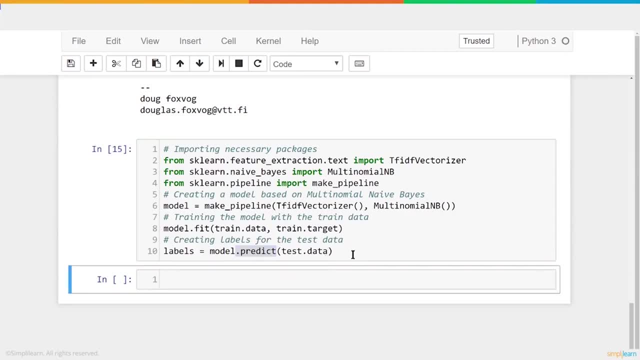 do they match what they should be? now? i've already read this through. there's no actual output, so we're going to put our test data in there and we're going to put our test data in there and we're going to put it to it to show. this is just setting it all up. this is just training our 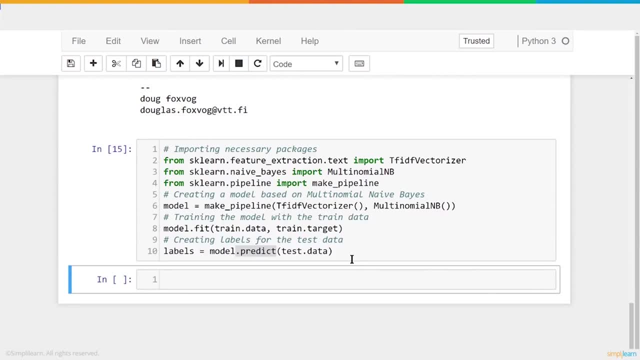 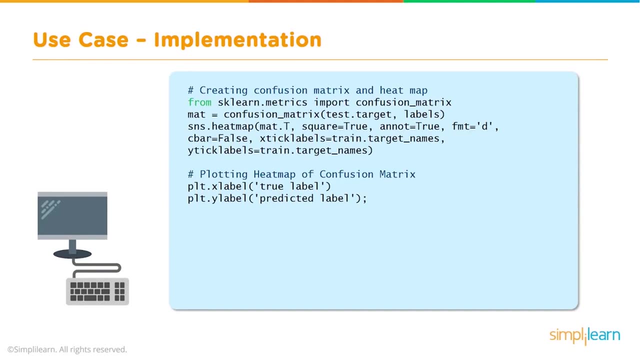 model, creating the labels, so we can see how good it is, and then we move on to the next step, to find out what happened. to do this, we're going to go ahead and create a confusion matrix and a heat map. so the confusion matrix, which is confusing just by its very name, is basically going to ask how 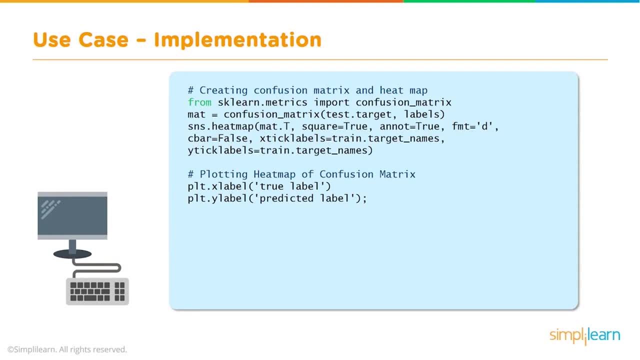 confused is our answer? did it get it correct or did it miss some things in there or have some labels? and then we're going to put that on a heat map, So we'll have some nice colors to look at to see how that plots out. Let's go ahead and take this code and see how that, take a walk through it and see what that looks like. 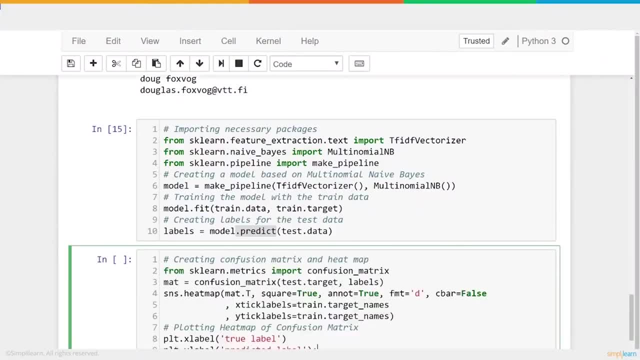 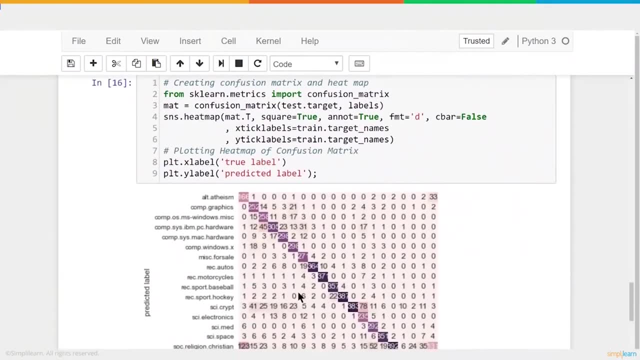 So back to our Jupyter notebook. I'm going to put the code in there And let's go ahead and run that code. Take it just a moment And remember we had the end line. That way my graph shows up on the end line here. 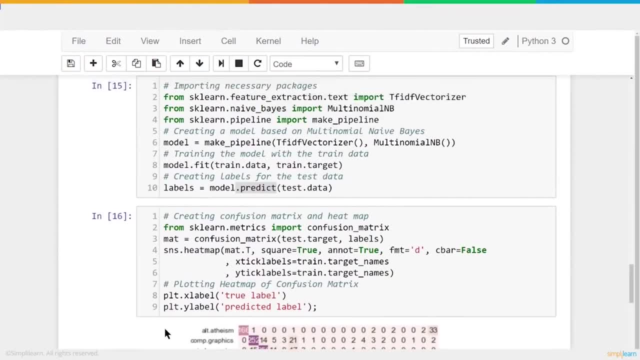 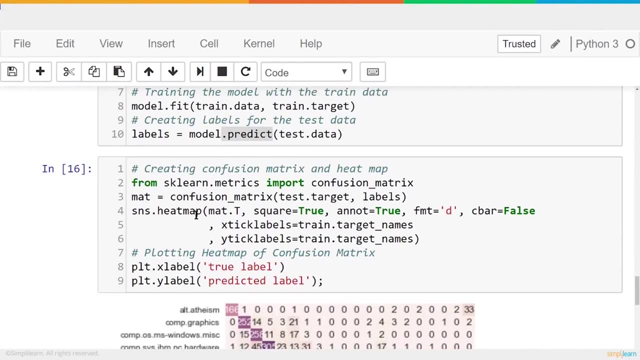 And let's walk through the code and then we'll look at this and see what that means. So let me get a little bit bigger. There we go, No reason not to use a whole screen Too big. So we have here from sklearnmetrics import confusion matrix. 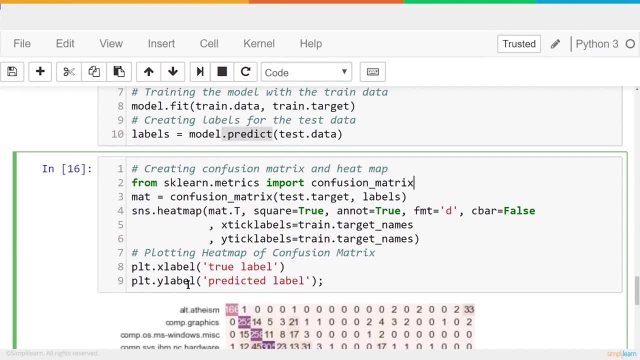 And that's just going to generate a set of data that says the prediction was such. the actual truth was either agreed with it or it was something different. And it's going to add up those numbers so we can take a look and just see how well it worked. 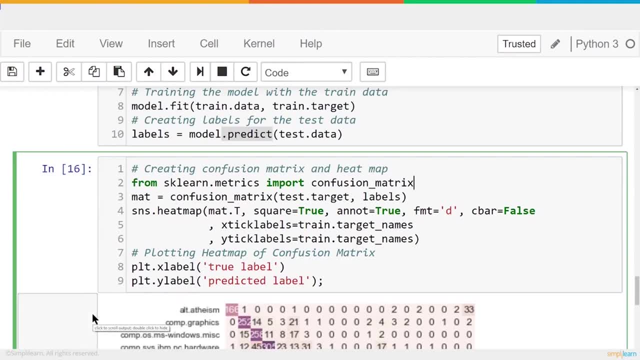 And we're going to set a variable mat equal to confusion matrix. We have our test target, our test data. that was not part of the training- Very important in data science. We always keep our test Data separate, Otherwise it's not a valid model if we can't properly test it with new data. 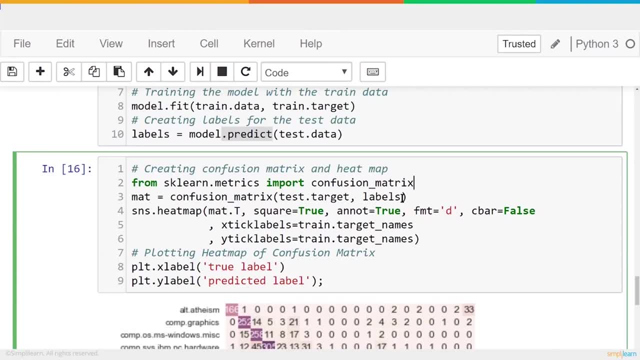 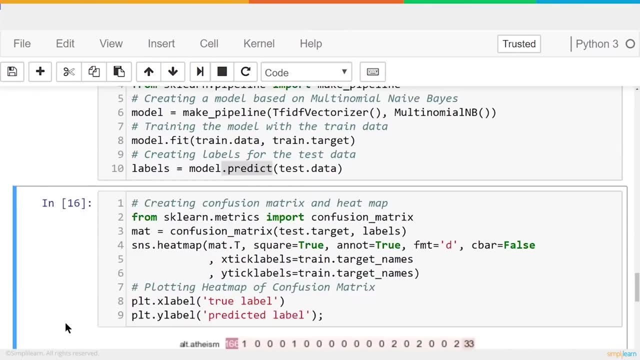 And this is the labels we created from that test data. These are the ones that we predict it's going to be. So we go in and we create our SN heat map. The SNS is our seaborne, which sits on top of the pi plot. 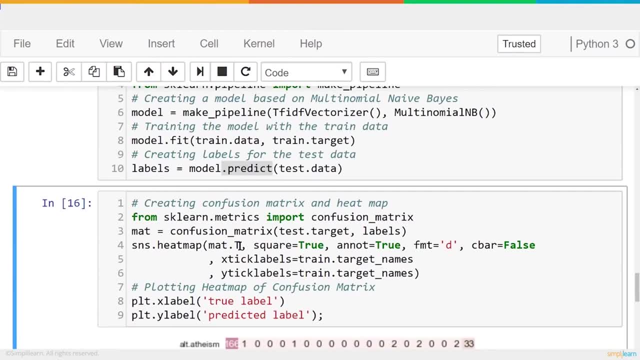 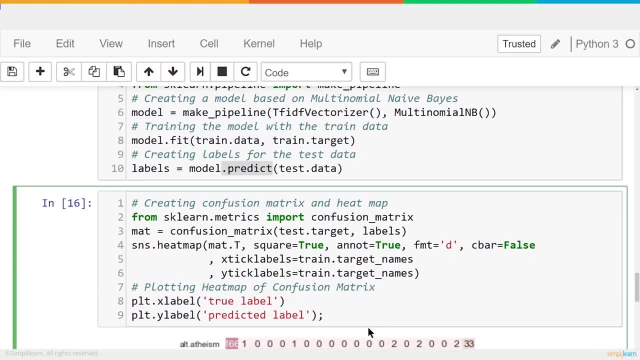 We're not going to go into detail what all the variables mean. We're not going to go into detail what all the variables mean. The annotation equals true, That's what tells it to put the numbers here. So you have the 166, the 1001.. 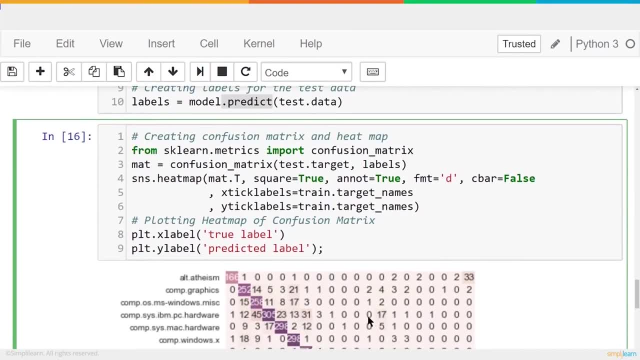 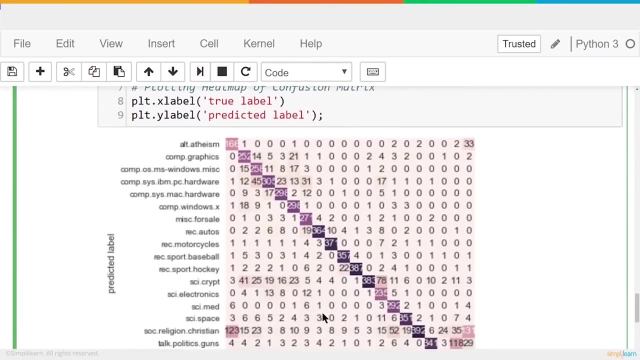 Format D and C bar equals false. Have to do with the format. If you take those out you'll see that some things disappear. And then the x tick labels and the y tick labels- Those are our target names And you can see right here that's the alt atheism comp graphics. 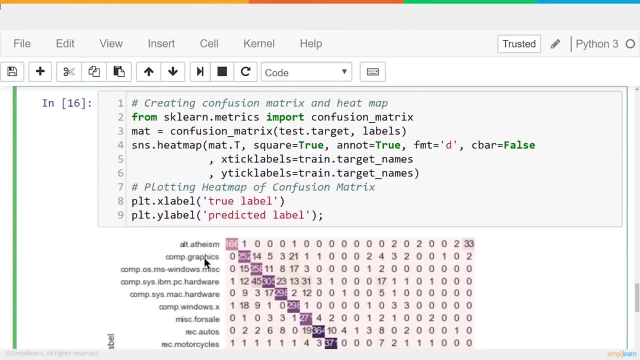 Comp OS, MS Windows, dot, miscellaneous. And then, finally, we have our parallel. And then, finally, we have our parallel, have our pltxlabel. Remember the sns or the seaborn sits on top of our matplotlibrary, our plt. and so we want to just tell it: xlabel equals a true is true, The labels are true. and then the 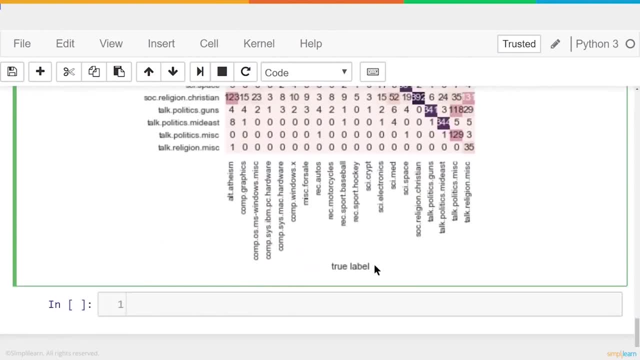 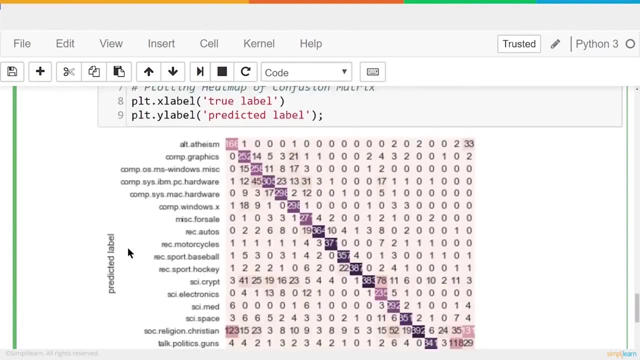 ylabel is prediction label. So when we say a true, this is what it actually is and the prediction is what we predicted. And let's look at this graph, because that's probably a little confusing the way I rattled through it, And what I'm going to do is I'm going to go ahead and flip back to the slides. 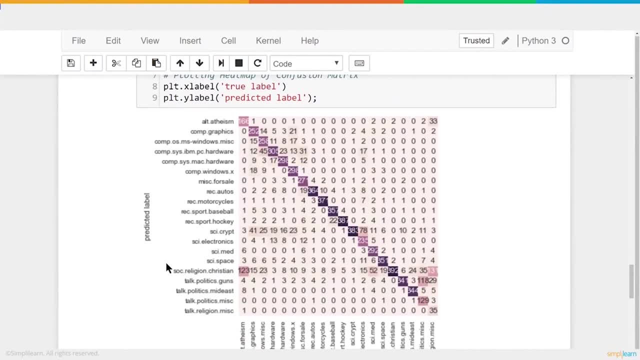 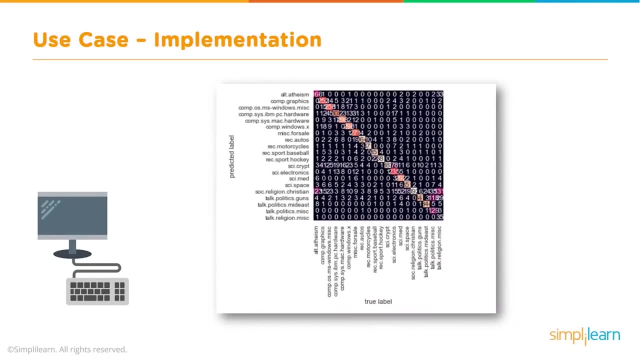 because they have a black background they put in there. that helps it shine a little bit better so you can see the graph a little bit easier. So in reading this graph, what we want to look at is how the color scheme has come out, And you'll see a line right down the middle, diagonally from upper 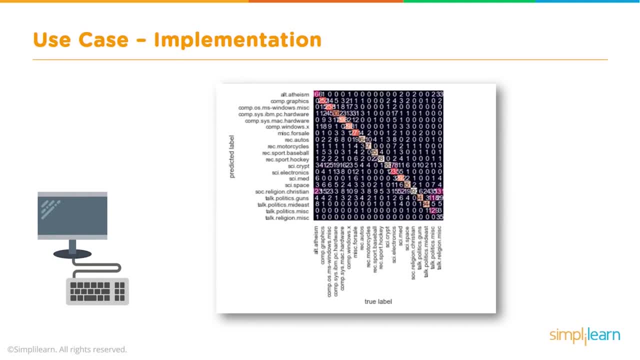 left to bottom right. What that is is, if you look at the labels, we have our predicted label on the left and our true label on the right. Those are the numbers where the prediction and the true come together, And this is what we want to see is we want to see those lit up. That's what that heat. 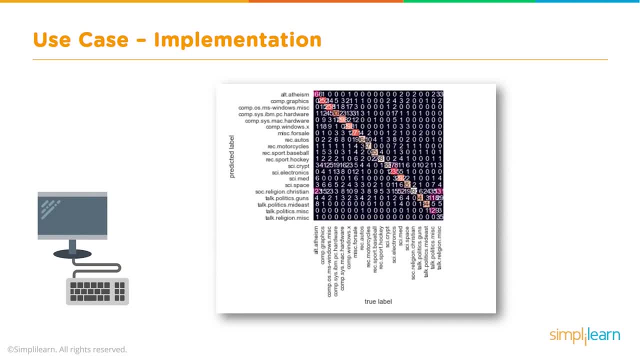 map is. So we want to see those lit up And we want to see those lit up And we want to see those red spots, And we want to see those red spots. And then you get an observation of what the heat map does. As you can see, it does a good job of finding those data And you'll notice that there's 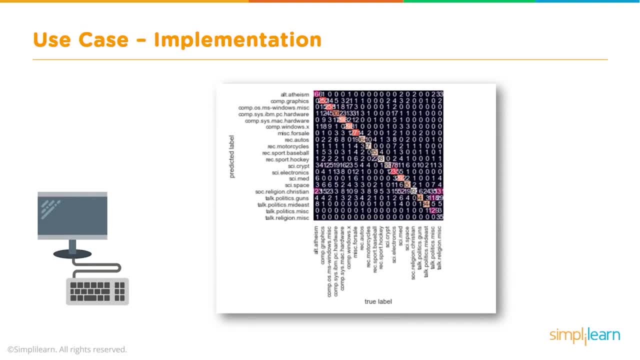 a couple of red spots on there where it missed. You know it's a little confused when you talk about talk religion, miscellaneous versus talk politics, miscellaneous Social religion, Christian versus alt atheism. It mislabeled some of those And those are very similar topics so you could. 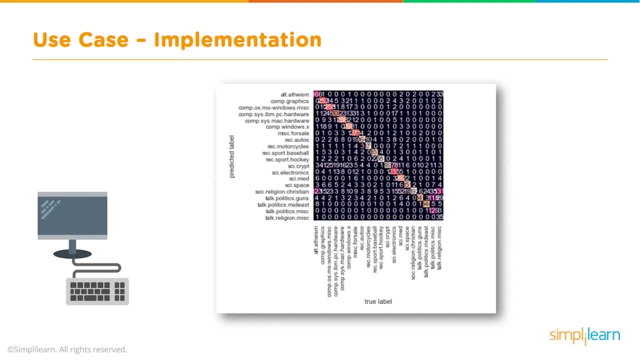 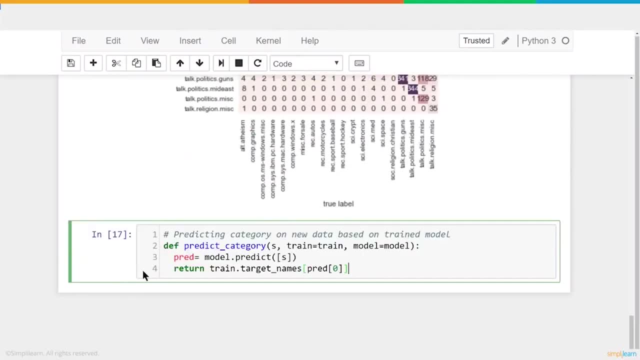 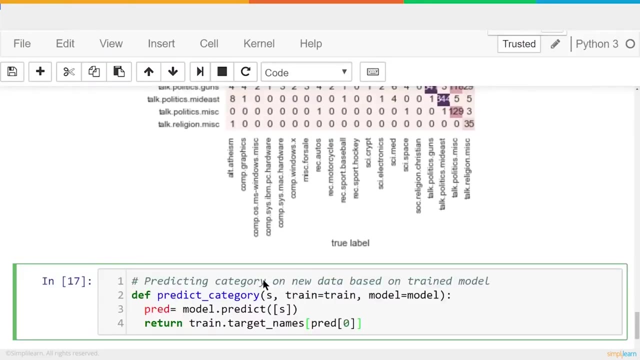 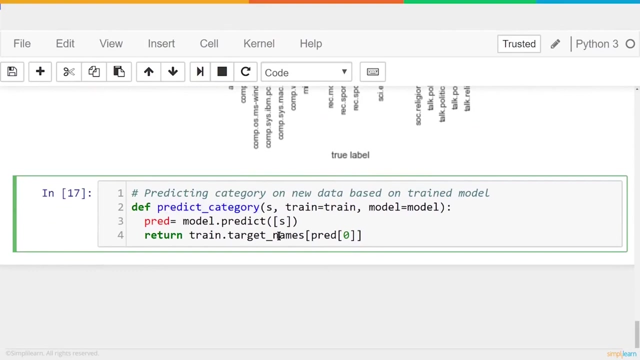 understand why it might mislabel them, But overall it did a pretty good job. If we're going to create these models, we want to go ahead and be able to use them. So let's see what that actually means, what that looks like. To do this, let's go ahead and create a definition, a function to run, and we're going to call this function. let me just expand that just a notch here. there we go. I like mine in big letters: predict categories. We want to predict the category. we're going to send it s a string and then we're sending it. train equals train. we have our training model and then we had our pipeline: model equals model. This way, we don't have to resend these variables each time. The definition knows that. because I said train equals train and I put the 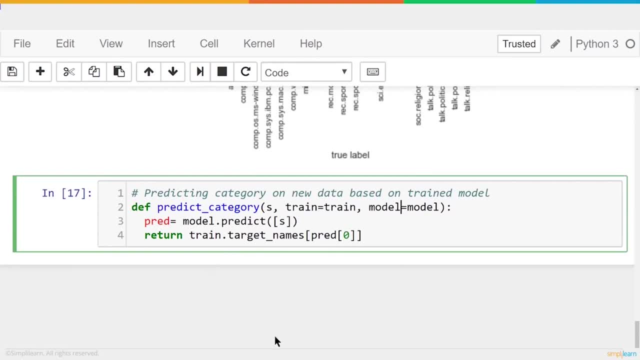 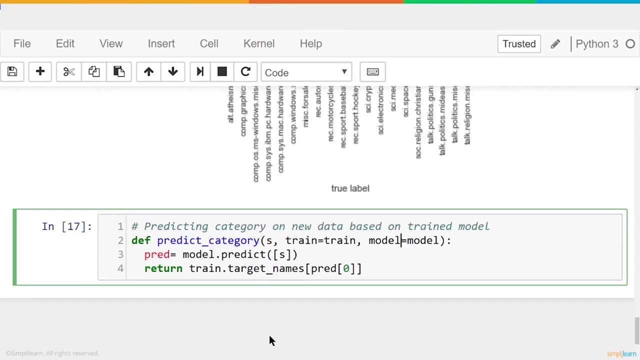 equal for model And then we're going to set the prediction equal to the modelpredict s. so it's going to send whatever string we send to it. it's going to push that string through the pipeline, the model pipeline. It's going to go through and tokenize it and put it through the tf, idf, convert that into numbers and weights for all the different documents and words, and then it'll put that through our naive bays And from it we'll go ahead and get our prediction. We're going to predict what value it is. 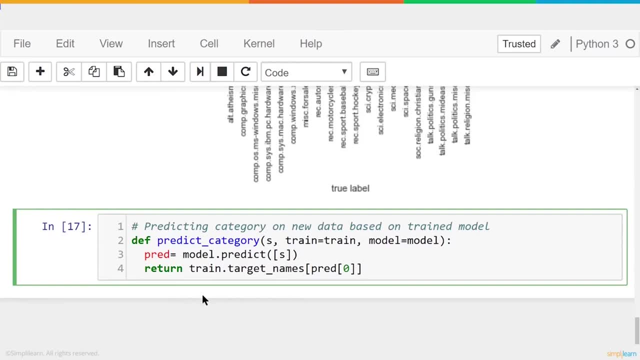 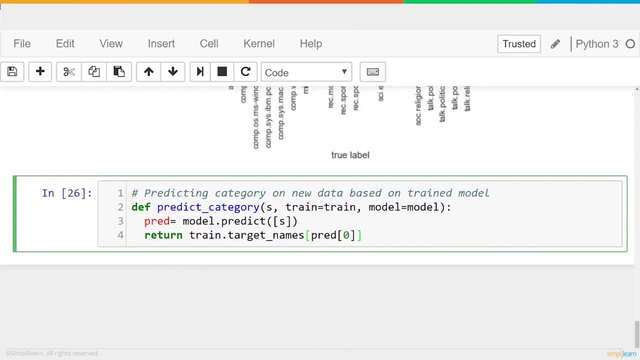 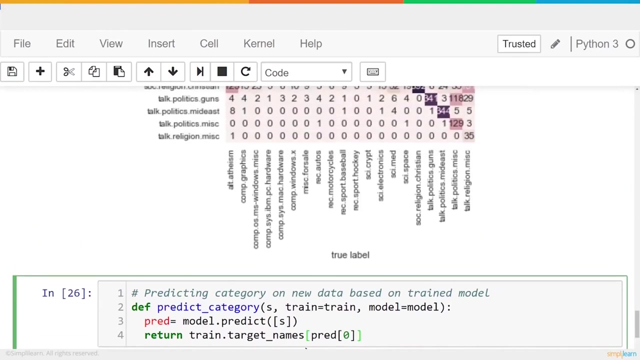 And so we're going to return traintargetNames- predict of 0. And remember that the traintargetNames, that's just categories. I could have just as easily put categories in therepredict of 0.. So we're taking the prediction, which is a number, and we're converting it to an actual category. We're converting it from. I don't know what the actual numbers are, but let's say, 0 equals alt atheism, so we're going to convert that 0 to the word, or 1, maybe it equals comp graphics, so we're going to convert number 1 to 0.. 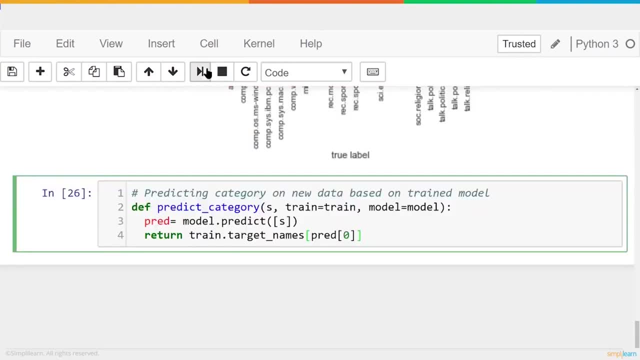 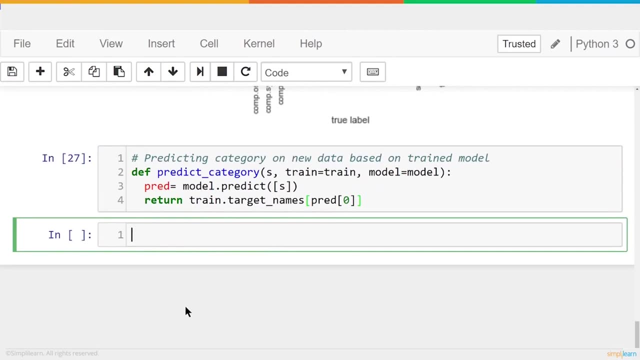 into comp graphics. that's all that is. and then we got to go ahead, and, and then we need to go ahead and run this, so I load that up and then, once I run that, we can start doing some predictions. let me go ahead and type in predict category. 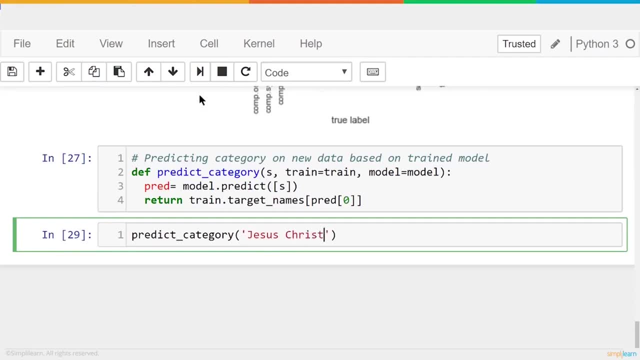 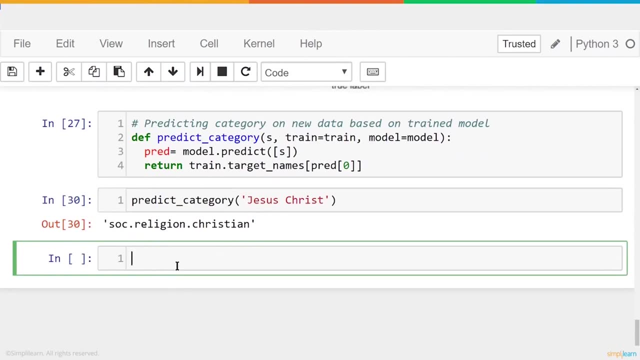 and let's just do predict category Jesus Christ and it comes back and says it's social religion Christian. that's pretty good. now note: I didn't put print on this. one of the nice things about the Jupiter notebook editor and a lot of inline editors is, if you just put the name of the variable out is returning the. 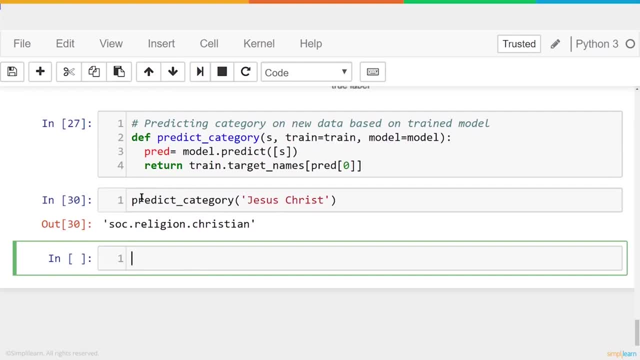 variable train dot target underscore names. it'll automatically print that for you in your own ID. you might have to put in print. let's see where else we can take this. and maybe you're a space science buff, so how about sending load to International Space Station? and if we run that we get science, space, or maybe? 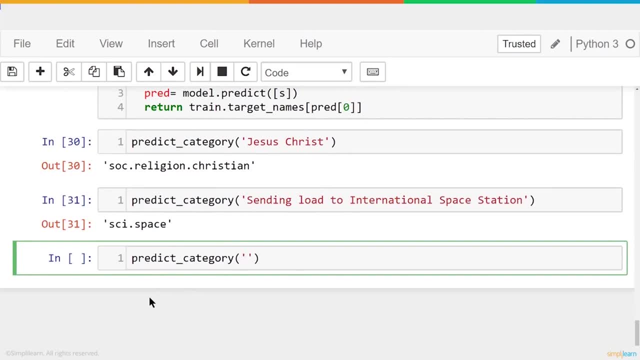 you're a call buff and let's do. they were going to tell me: Audi is better than BMW, but I'm going to do: BMW is better than an Audi. so maybe you're a car buff and we run that and you'll see. it says recreational. I'm assuming that's what REC stands for. 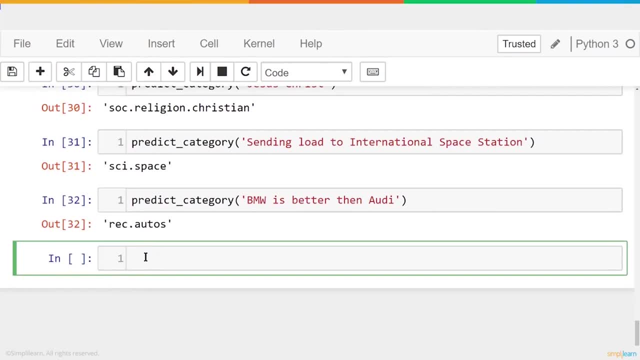 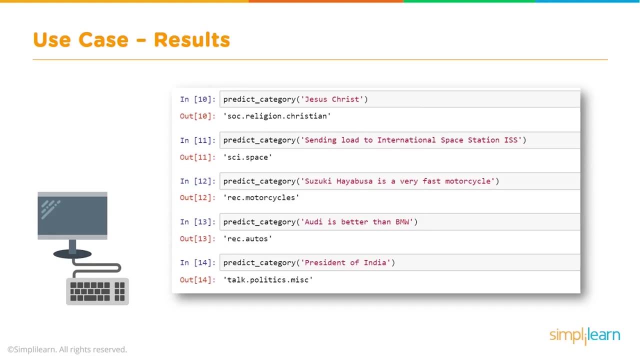 autos. so I did a pretty good job labeling that one. how about if we have something like a caption running through their president of India and if we run that it comes up and says: talk politics miscellaneous. so when we take our definition, our function and we run all these things, 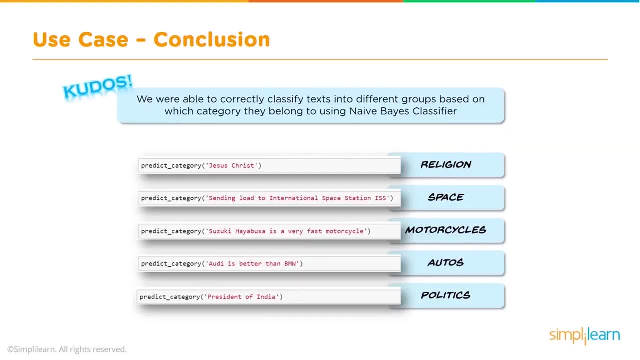 through kudos. we made it. we were able to quickly classify text into different groups based on which category they belong to, using the naive Bayes classifier. now we did throw in the pipeline the TF idea vectorizer. we threw in the graphs. those are all things you don't necessarily have to know to 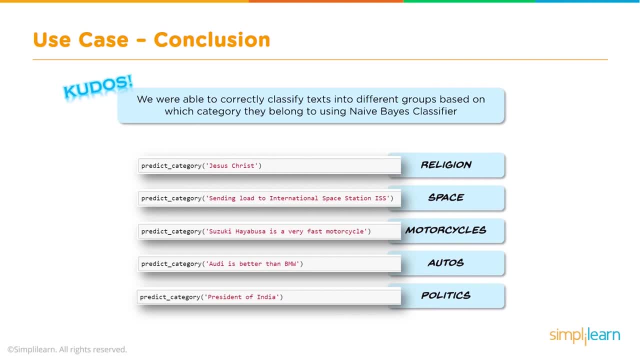 understand that the naive Bayes setup or classifier, but they're important to know. one of the main uses for the naive Bayes is with the TF, IDF tokenizer vectorizer, where it tokenizes a word and as labels, and we use the pipeline because you need to push all that data through and it. 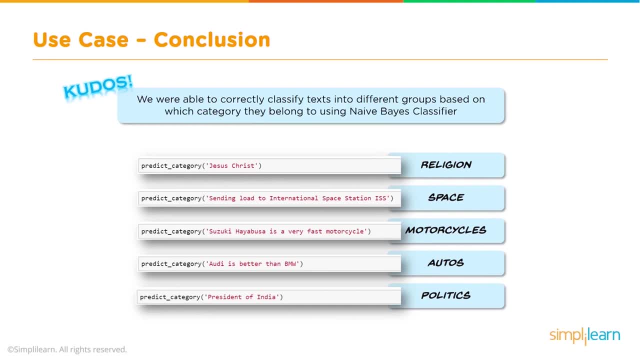 makes it really easy and fast. you don't have to know those, understand naive Bayes, but they certainly help for understanding the industry and data science. and we can see our categorizer, or naive Bayes classifier. we were able to predict the category: religion, space, motorcycles, autos, politics- and properly. 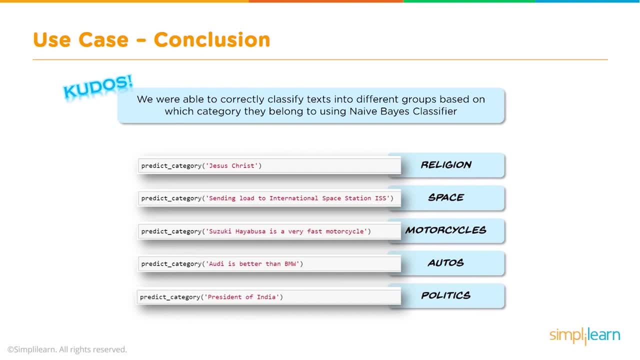 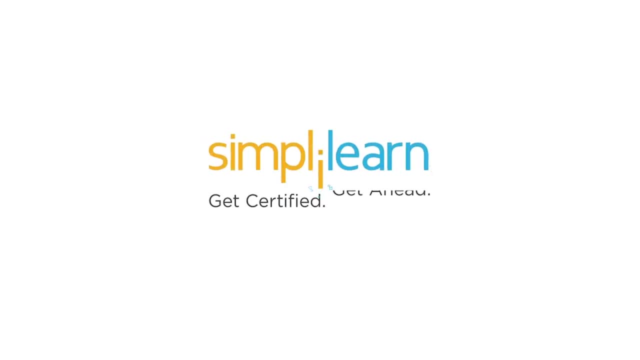 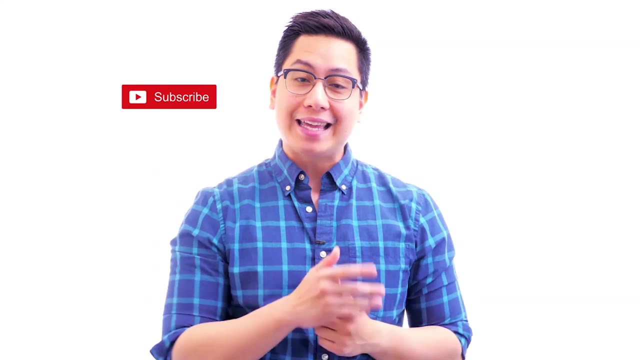 classify all these different things we pushed into our prediction in our train model. hi there. if you like this video, subscribe to the simply learn YouTube channel and click here to watch similar videos. to nerd up and get certified: click here.